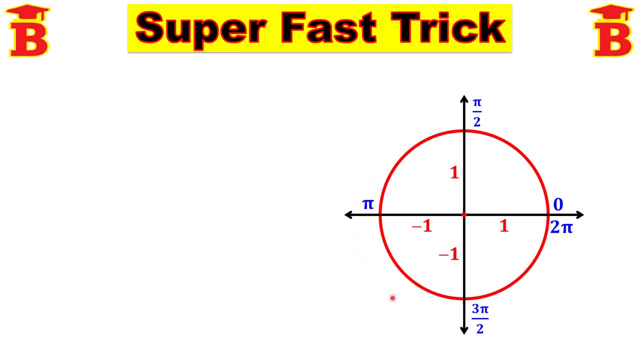 Next 3 pi and then 7 pi by 2 and then 4 pi. This is second rotation. Similarly, we can continue the angles. And now, for sign values, we have to take the vertical line, And for cos values we have to take the horizontal line. 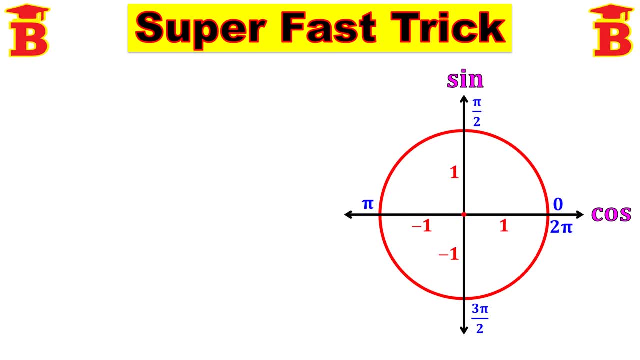 So for sign values we have to take the rising distance, that is vertical line, And for cos values we have to take the running distance, that is horizontal line. Now from the diagram it is clear that the sign values exist only for the vertical angles. 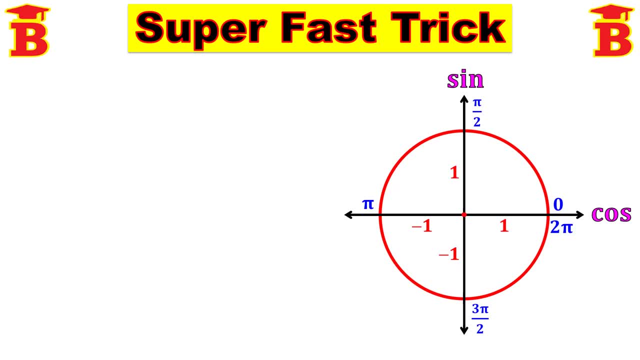 that is, pi by 2,, 3, pi by 2 and other similar angles, And the cos values exist only for 0, pi, 2, pi and similar angles. Now we can write all the values. Sign value exists only for pi by 2,, 3, pi by 2 and so on. 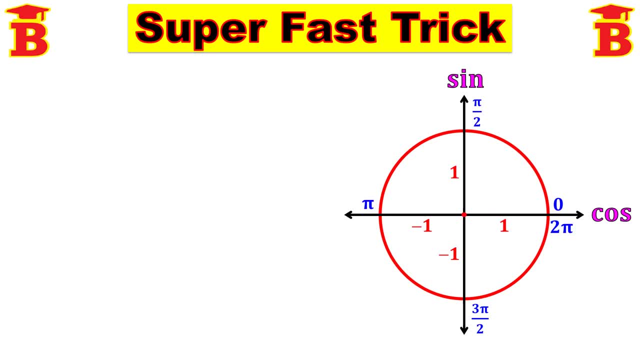 That means for horizontal line sign value is 0. So horizontal angle is 0, pi 2, pi, 3, pi, 4, pi, etc. For all these sign value is 0. That is sign 0, 0,, sign pi 0,, sign 2, pi 0,, etc. 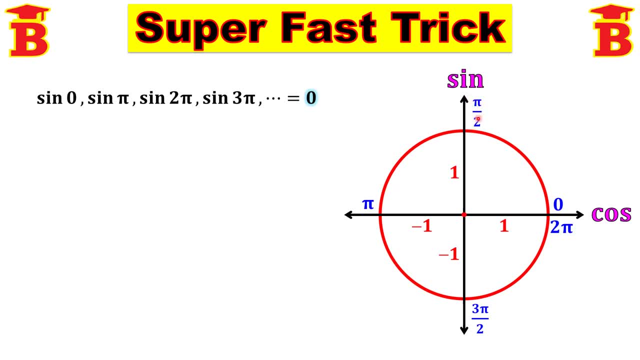 And sign value. on the positive side we have pi by 2. And after rotation we have 5 pi by 2, and again 9 pi by 2, etc. For all these we have the value plus 1.. So positive side plus 1.. 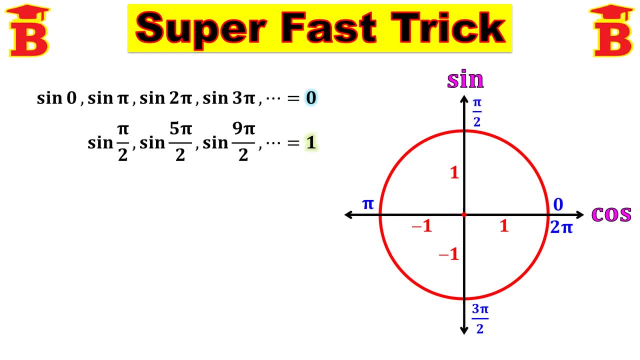 Negative side minus 1.. Positive side angles are: pi by 2, 5, pi by 2, 9, pi by 2, etc. That is, sign pi by 2, 1, sign 5 pi by 2, 1,, sign 9 pi by 2, 1,, etc.